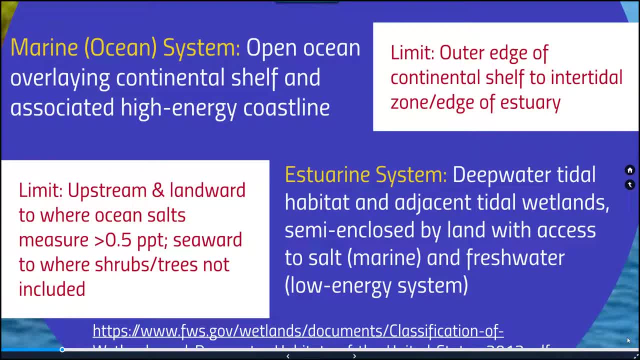 The estuary system kind of takes over from there and it's the deep water, tidal habitat and adjacent tidal wetlands that is semi-enclosed by land and has access to salt water or marine water and fresh water. These tend to be lower energy systems. 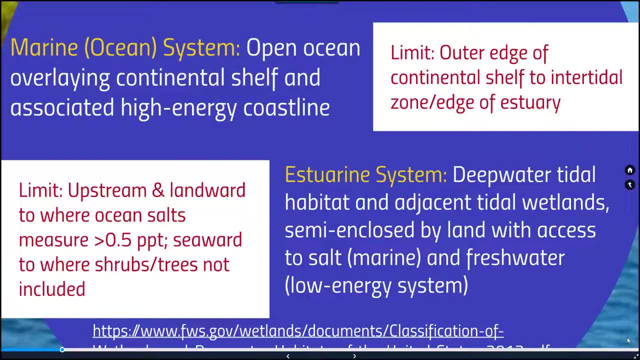 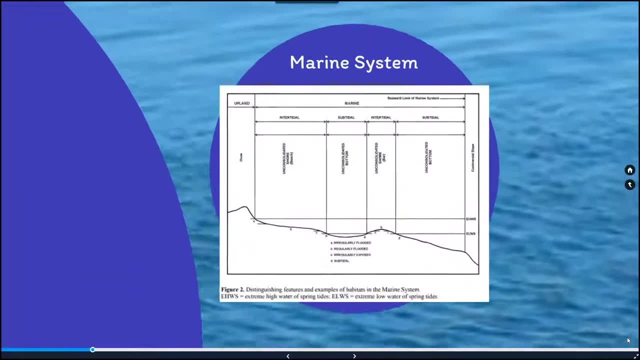 The limit of these estuarine systems are the upstream and landward areas where the ocean salts measure less than 0.5 parts per thousandth. The seaward element is where the shrubs and the trees are not included. So just to give you a couple graphics on these different wetland regions. 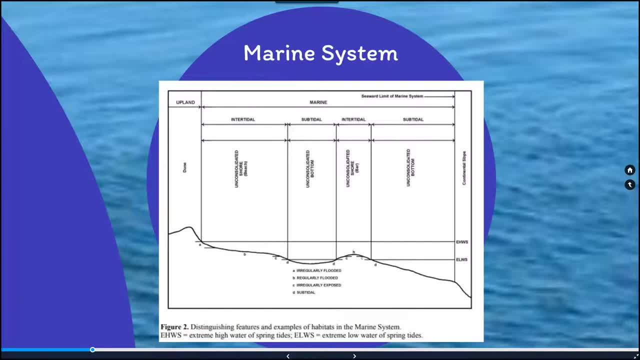 Here we have the continental slope located at the right edge of this figure. Here we have the continental slope located at the right edge of this figure, And over on the left hand side of this figure we have a dune region along the shore. So somewhere along here from that dune down to about here or so, is where we have that inner tidal region. 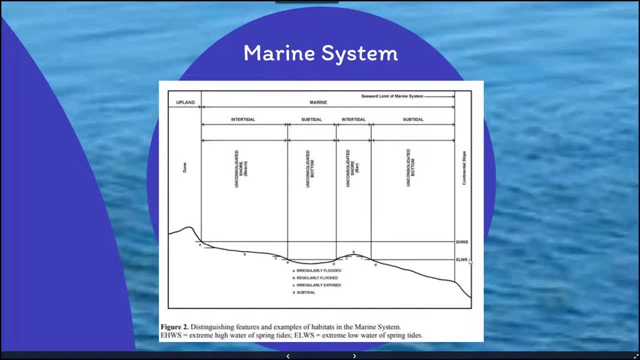 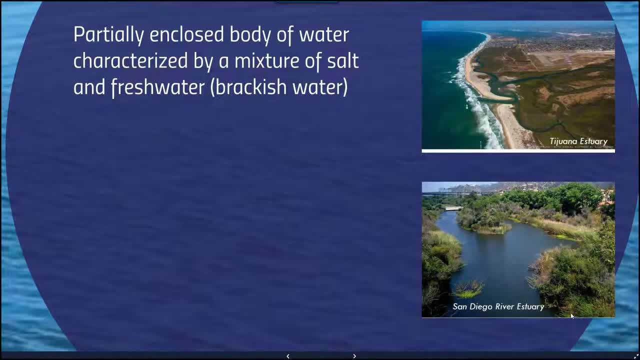 our county and on the bottom here, the San Diego River estuary. so there's variability in terms of the how, those, the layout and whatnot of those different estuaries. there's a zone of they're considered a zone of transition between the land and the ocean and they're going to be typically influenced. 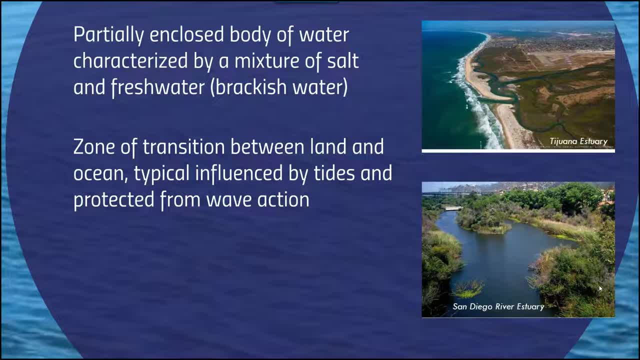 by tides and protected from wave action which is going to constitute or be a little bit more active in that marine wetland region. estuaries can either be referring to or kind of corresponding to bays, lagoons and harbors and sounds and are often- these terms are often used interchangeably to describe estuaries. so 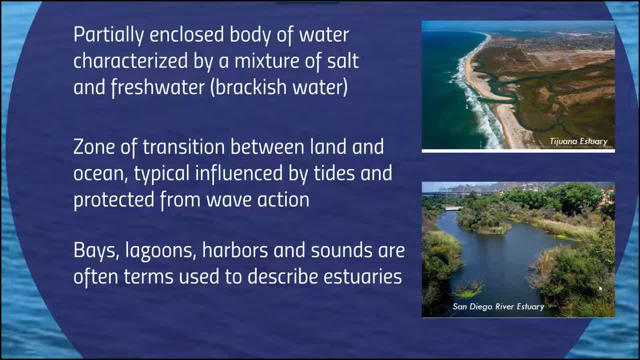 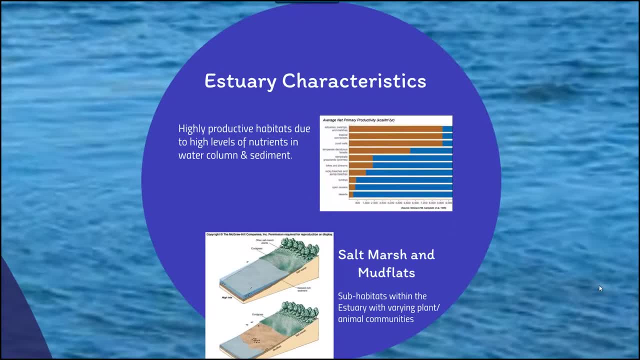 you'll see a bit of variability in terms of the- either the naming convention of a particular estuary or how it's referred to by individuals. as you can see, here, there's a little bit of variability in terms of the- either the naming convention of a particular estuary or how it's referred to by individuals. as 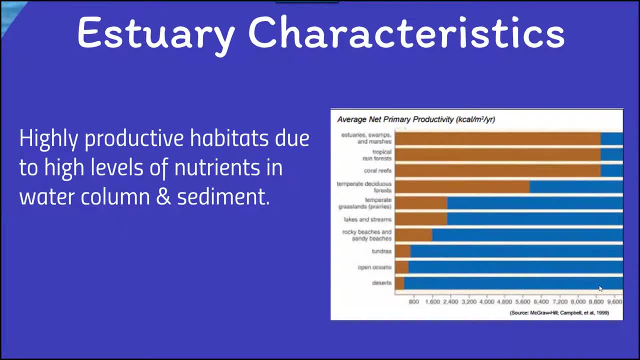 estuaries are highly productive habitats due to high levels. of estuaries are highly productive habitats due to high levels of nutrients in the water column and in the sediment. so, as you can see in this, nutrients in the water column and in the sediment. so, as you can see in this, 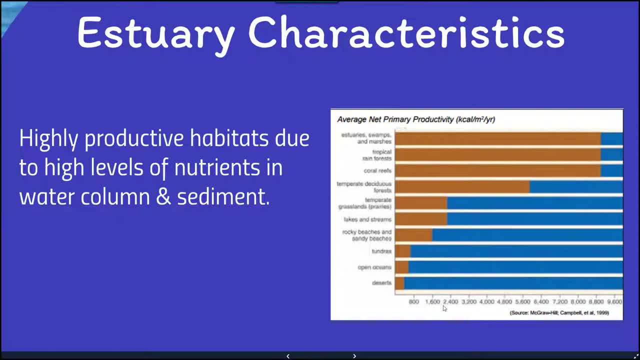 figure to the right hand side, we have the net primary productivity along the x-axis calculated as kilo cows per meter squared per year, and then we have several different categories of marine as well as as wetland kind of regions, and also some terrestrial regions as well. so the 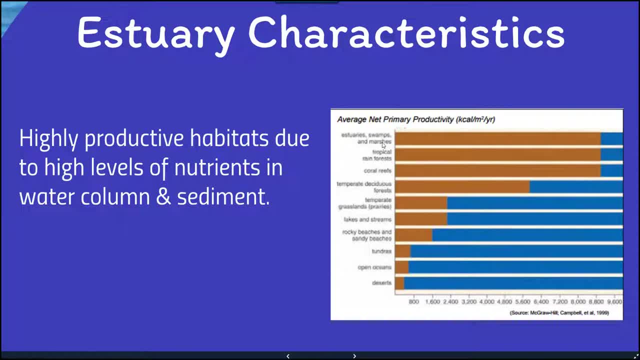 The estuary swamps and marshes that we're referring to here now have a comparable level of net primary productivity to tropical rainforests and coral reefs. So, as you can imagine, that makes them incredibly important regions and habitats that we'll feed into and whose nutrient cycles will contribute to surrounding habitats and ecosystems. 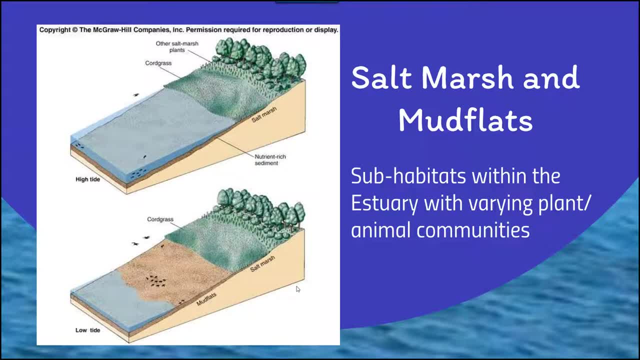 Salt marshes and mudflats tend to have this sub habitat or sub habitats within the estuary and within these kind of riverine and lacustrine systems. Estuaries are going to vary with respect to the plant and animal communities, So each individual estuary that you find can have a very unique diversity and assemblage of organisms, which makes them so incredibly important as well. 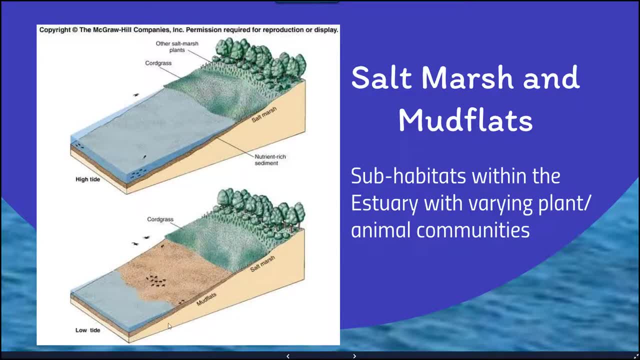 In this particular figure off to the left hand side, we have an example of just a salt marsh, where you have the nutrient rich sediments and water that lead right up to a segment or section of grass, some type of seagrass, as well as salt marsh plants. 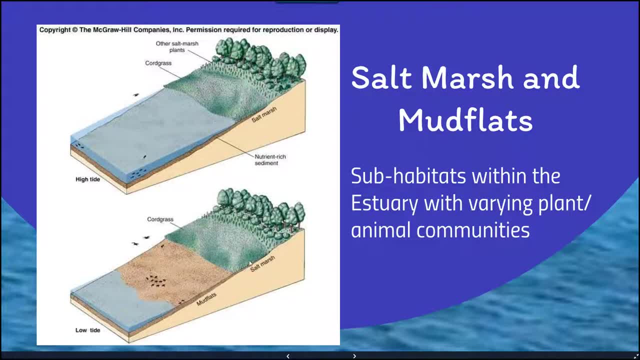 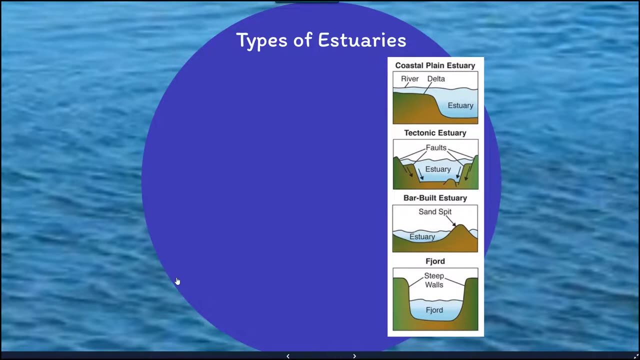 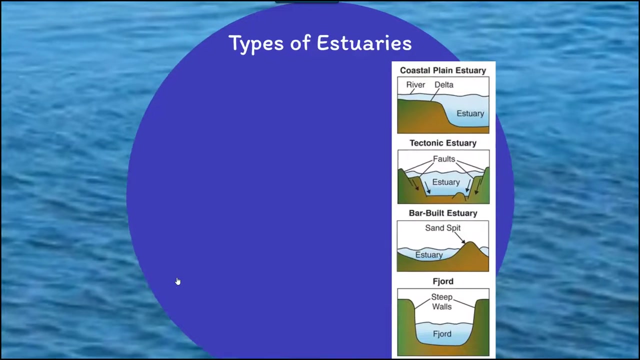 Whereas a mudflat, you'll have a segment just in between the vegetation area and the waterline that consists of just kind of a very nutrient rich mud that a lot of organisms tend to exist in. There are several different forms or types of estuaries in terms of the topographical features that are going to form them. 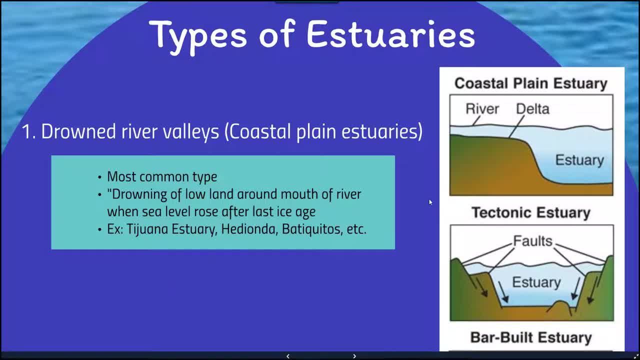 The drowned river valleys or the coastal plain estuaries which are demonstrated or depicted in this figure in the upper right hand side are going to be the most common type that are encountered And, essentially, the drowning of lowland around the mouth of the river when the sea level rose after the last ice age is what kind of estuary that I've drawn here. And so the most common estuaries would be the salt marshes in the back of the estuary and the mudflats. And so the most common estuaries would be the salt marshes in the back of the estuary and the mudflats. 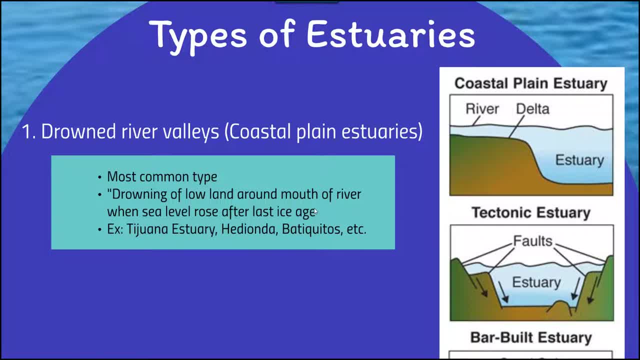 form. these Examples of these in San Diego include the Tijuana estuary, Hedionda, Barraquitos, there's a couple others within San Diego County And here you can see we have a river with Delta which is going to be sediment, that's. 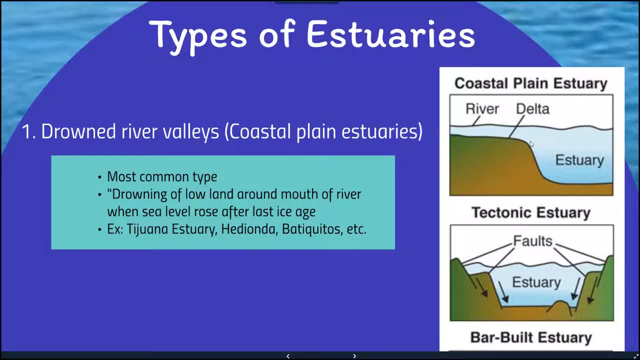 built up over time as the output, as it kind of follows down the river and is deposited at the mouth of that river and then the estuary kind of forms. just below that, Tectonic estuaries can also form, as you can see in the right hand. 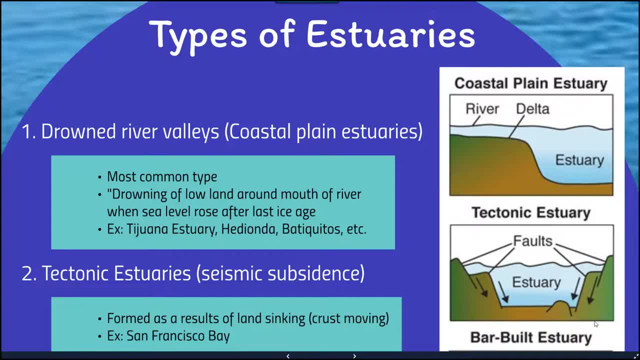 side here which they're going to form as a result of land sinking and the crust moving. So you have the crust of the earth that can, at these convergence points, it's going to shift and change around and that's going to form these different reservoirs of water that that will be. 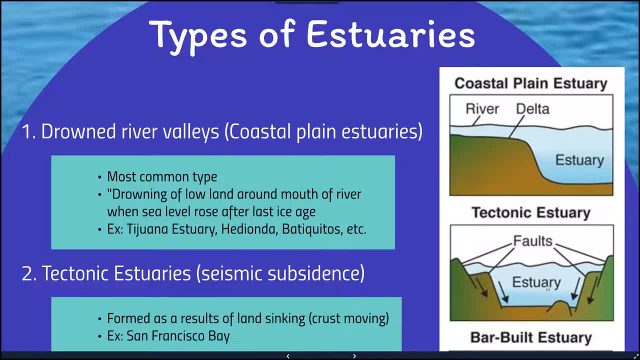 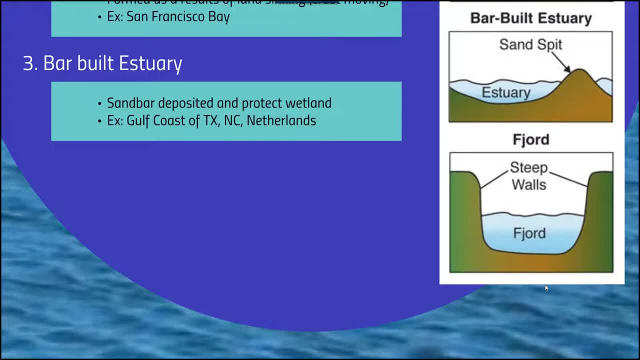 characteristically described as an estuary. A good example of this would be San Francisco. And moving to the other two types, we also have a find bar, built estuaries, which are sand bars deposited and protected wetlands. So you've got a sand. 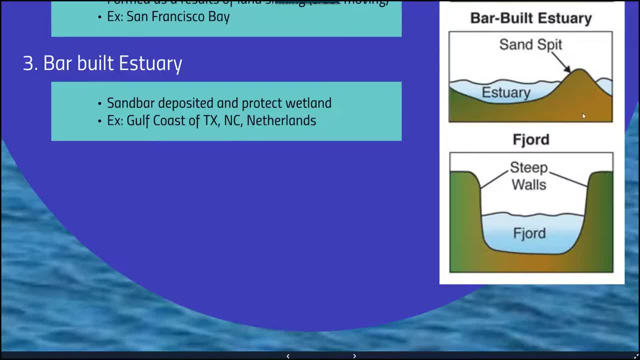 bar that results from deposition of some sediment and the built-up of that sediment over time, and as that increases in size, it will cut off access to the salt water there or the ocean water there. and well, there'll be some. it'll just act as a barrier. 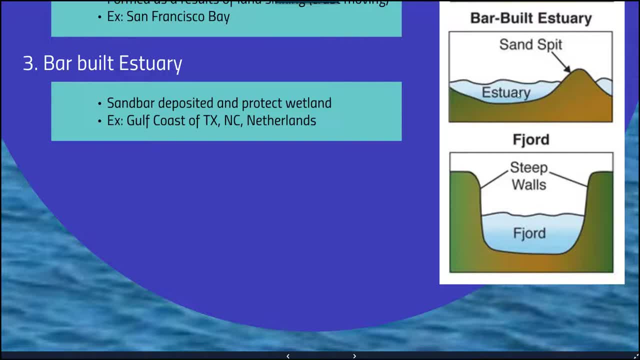 It won't be completely excluded, because otherwise it wouldn't be an estuary and it'll just kind of form this little reservoir. Good examples of this are the Gulf Coast of Texas, North Carolina and in the Netherlands. And then we have fjords which are going to be deep channels, cut in the coastal zone as a 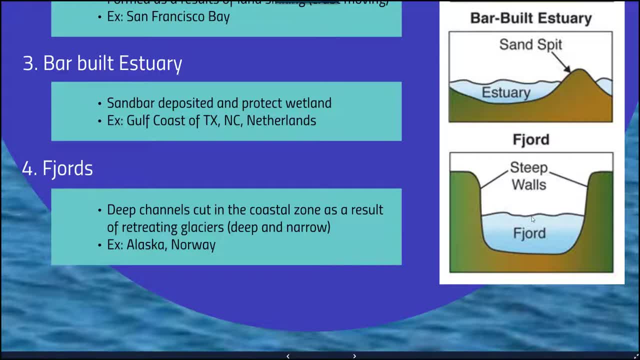 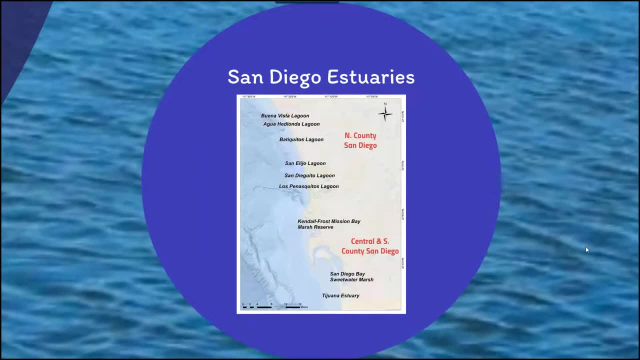 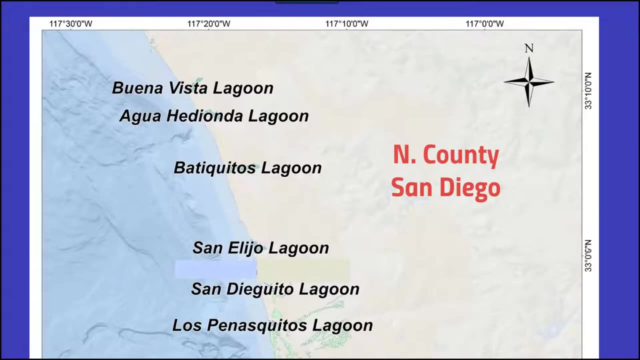 result of retreating glaciers. These tend to be really deep and narrow, and we find examples of these in Alaska and Norway. San Diego is home to several different estuaries. In the North County we find several different lagoons, a series of different lagoons along the coast and, sadly enough, 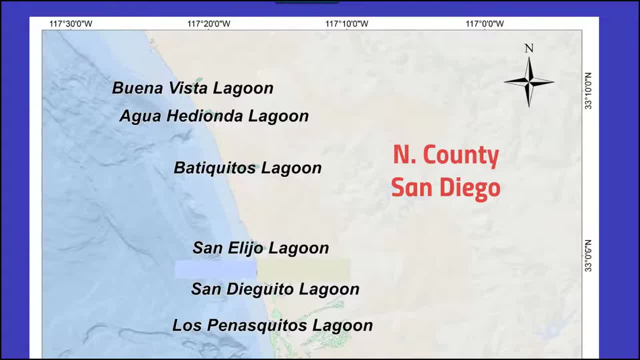 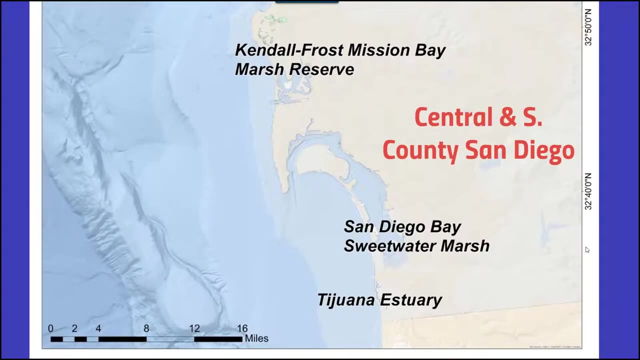 these lagoons have been kind of whittled down through development, as well as other, you know other kind of anthropogenic influences have been whittled down to these small areas. However, we still do have these and they are protected lands. In the southern part of San Diego County we have the Kendall 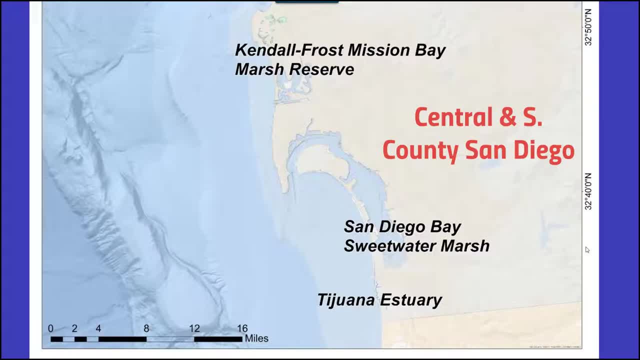 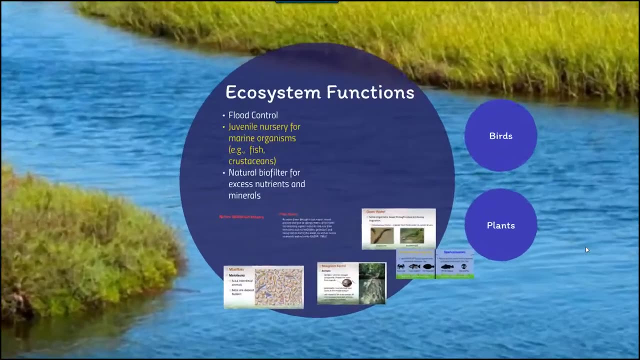 Frost, Mission Bay Marsh Reserve. so you probably visited that at Mission Bay and had the chance to check out some of those marshes up close: The San Diego Bay, Sweetwater Marsh and the Tijuana Astuary. Communities of organisms are going to find these ecosystems. 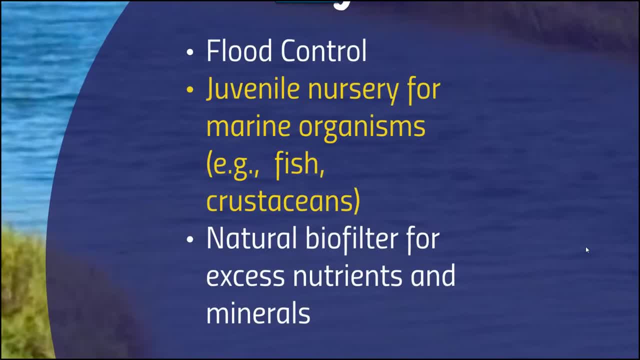 incredibly important. There are several different characteristics that are inherent to these different estuaries. First is the fact that they offer flood control, So flooding of these different habitats from offshore rivers is going to be retained and captured within that estuary. It's going to have some flood control there. 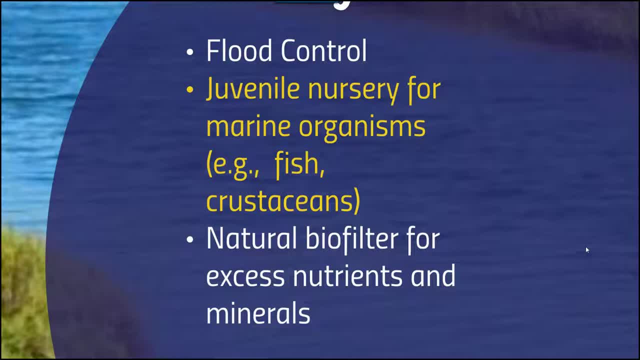 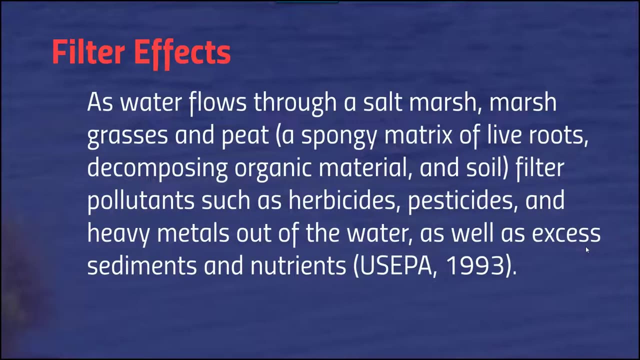 These estuaries serve as the juvenile nursery for many marine organisms, including fish and cetaceans. They also act as a natural biofilter for excess nutrients and minerals being deposited from the river system. So just an example of the filter effects As water flows through a salt marsh, marsh grasses and the peat. 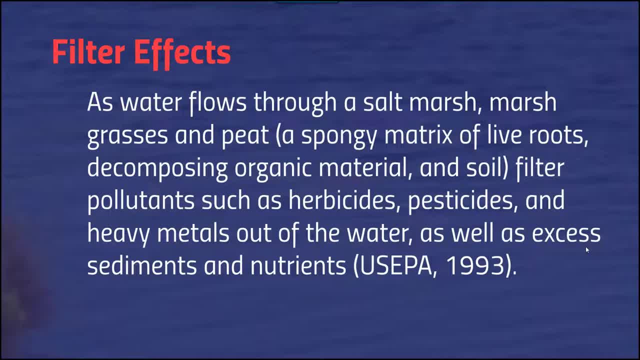 that's a spongy mix of live roots and decomposing organic material and soil are going to filter out pollutants such as herbicides, pesticides and heavy metals. This also will deal with excess sediments and nutrients. This is just a description of how that filtering works within that marshland or within that wetland. 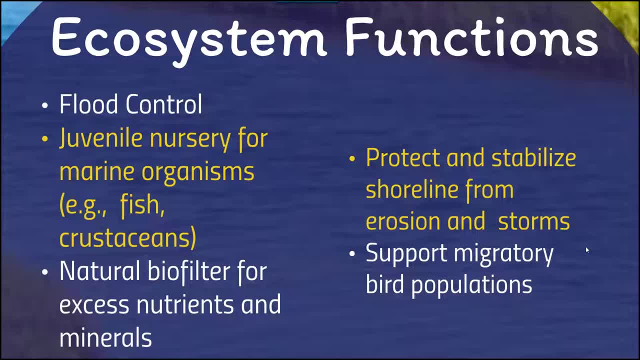 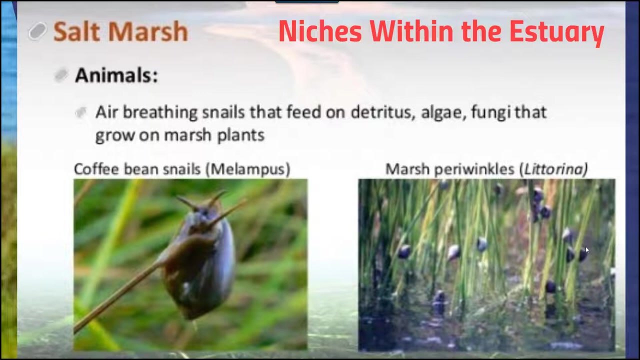 Another characteristic or kind of function of these ecosystems is their protection and stabilization of the shoreline from erosion and storms. They're also responsible for supporting migratory bird populations and a wide diversity of those birds as well. We find that there's different niches within the estuary, So, for example, some organisms are going to be air breathing and need to feed under. 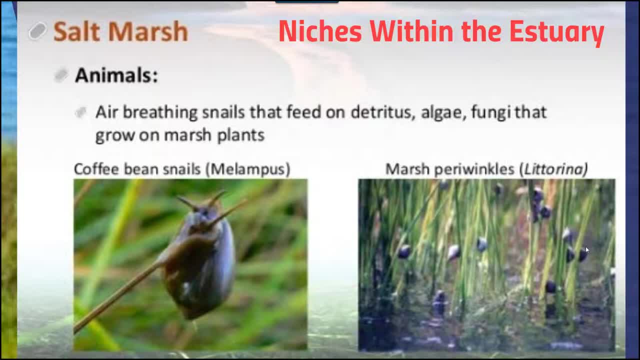 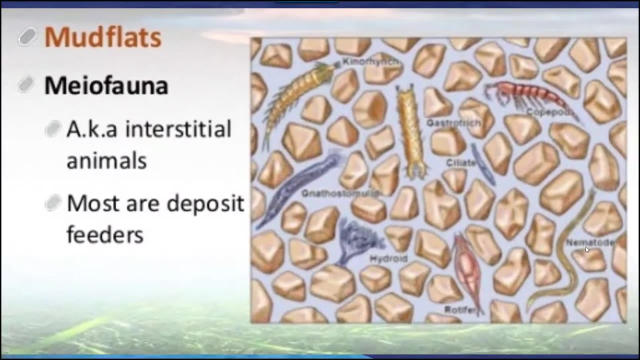 detritus, algae and fungi that grow on the salt marsh, plants, such as this coffee bean snail on the left hand side and the marsh periwinkles on the right hand side. So this is just one kind of section of the marshland that these organisms tend to inhabit. 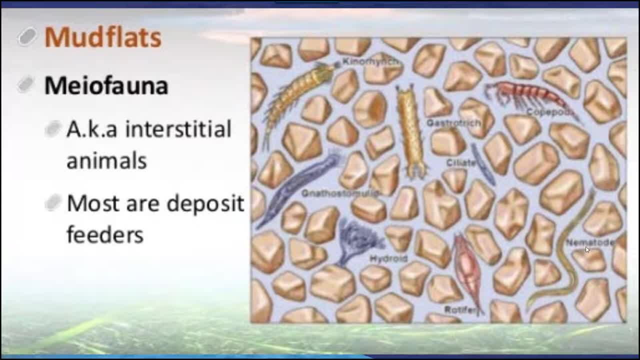 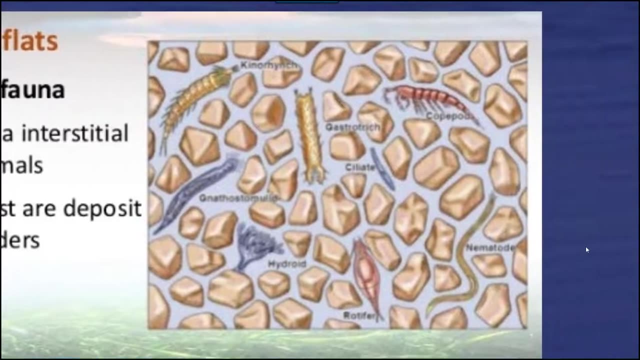 Whereas the mud flat areas are going to be inhabited by myofauna, so interstitial organisms or animals such as worms and ciliates and copepods that are going to be feed along the detritus and other materials that are found within those different sediments. 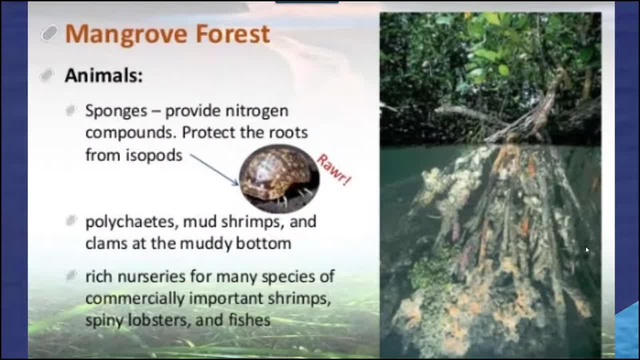 And then within a mangrove forest, we find something slightly different. So within the mangrove forest, we have animals such as sponges that provide nitrogen compounds and protect the roots from isopods. There's polychaetes, as well as mud shrimp and clams in the muddy bottom and a rich nursery of many different species. 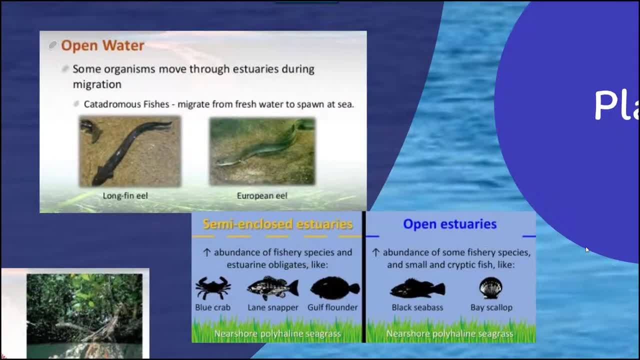 Within the open water regions of the estuary, often times we find catadromas, fishes which are going to be fish that migrated from fresh water to spawn in the sea. So an example is the longfin eel here, as well as the European eel, but also a good example would be salmon. 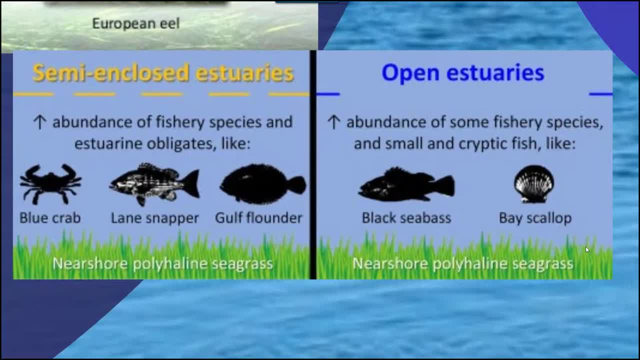 Within the estuaries you can have either a semi enclosed estuary where there's going to be access to the sea water, but there will also be regions that protect more from that wave action and kind of make the entrances to that seawater kind of smaller, And in those different estuaries there's an increased abundance of. 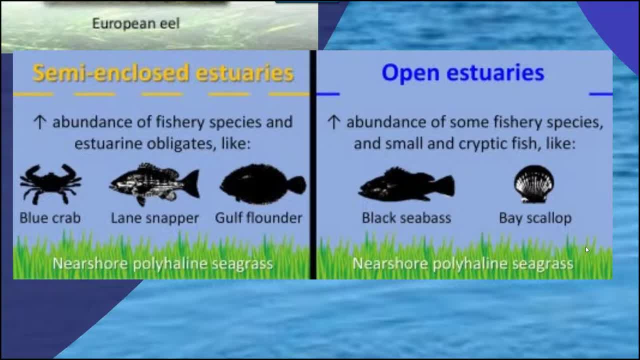 fish species or organisms such as blue crabs, snappers and gulf flounders. In the open estuaries, where there isn't that barrier or intermittent barrier occurring due to sandbars or things like that, you find a greater abundance of other fish and species, such as base gallops. 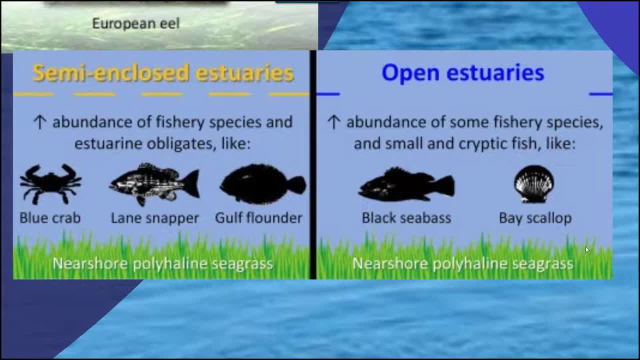 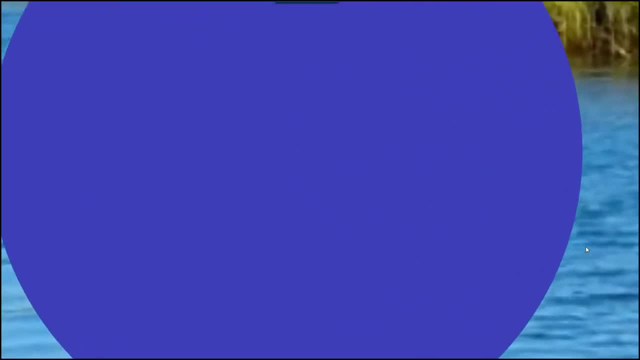 and black sea bass, So the assemblages and diversity of organisms are going to vary depending on the opening and access to that seawater as well. Estuary birds have a quite large diversity as well. In the coastal wetland we have migratory as well as resident species, And just to give you an idea of 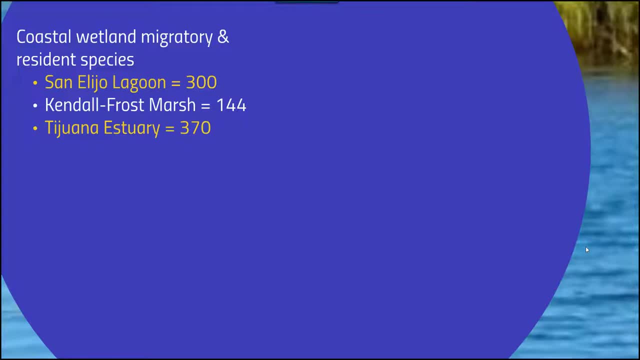 the diversity in these different regions. in San Diego, in Santa Lea Lagoon, there's approximately 300 species that either migrate to these lagoons or are residents. In the Kendall Frost Marsh, there's 144 different species, And then Tijuana estuary. 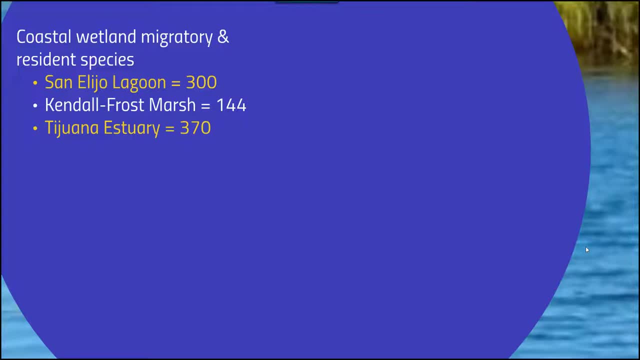 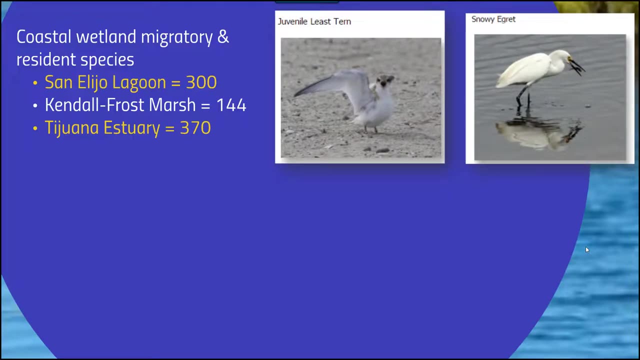 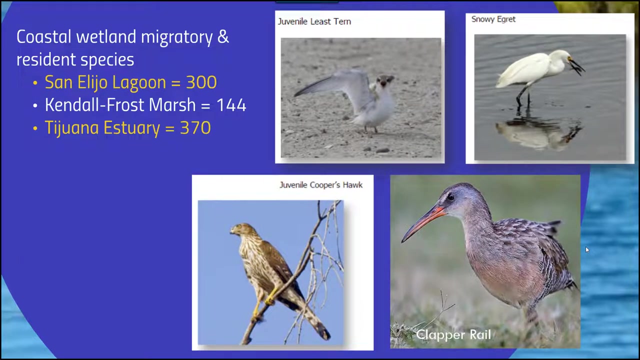 which I mentioned is the largest estuary in San Diego, has approximately 370 species of bird that rely on it. These include species such as the juvenile least tern and the snowy egret. Additionally, we find more predatory species such as the juvenile or, sorry, the larger prey. 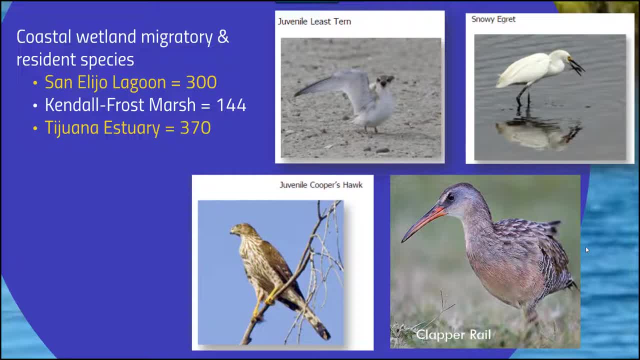 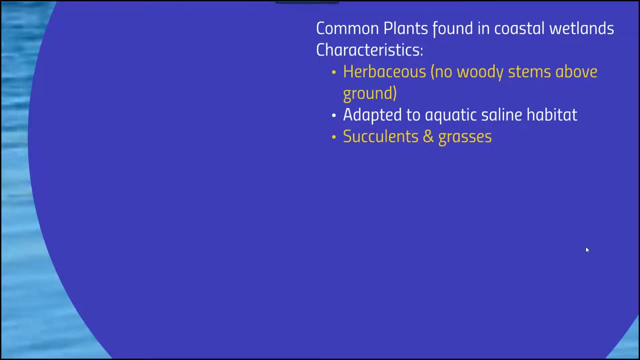 predators such as the juvenile cooper's hawk and the clapper rail Plants are also an interesting and diverse assemblage within these regions. There are several different common plants found in coastal wetlands. Their characteristics include the fact that they are herbaceous. 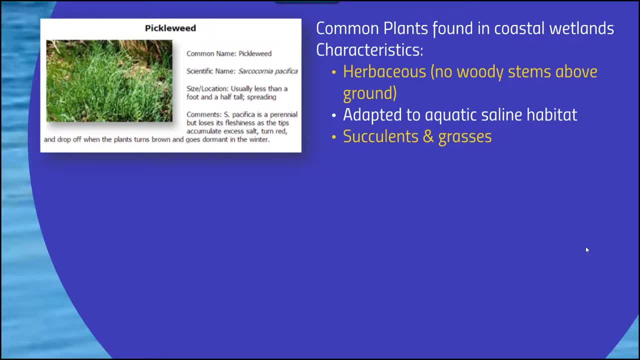 so there's no woody stem. They also have a lot of roots above the ground to make them a little bit lighter, so they don't have to have as an extensive or solid foundation. They're adapted to aquatic saline habitats and oftentimes they're going to consist of succulents and grasses. So off to the left-hand. 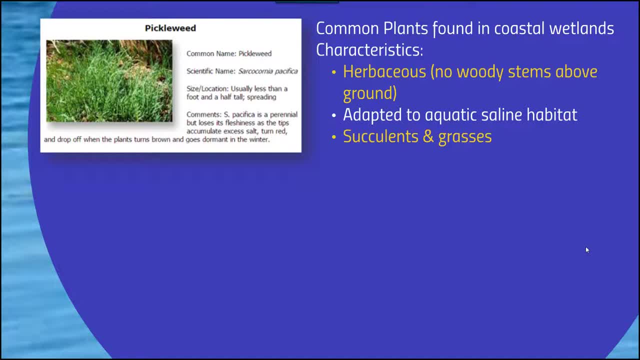 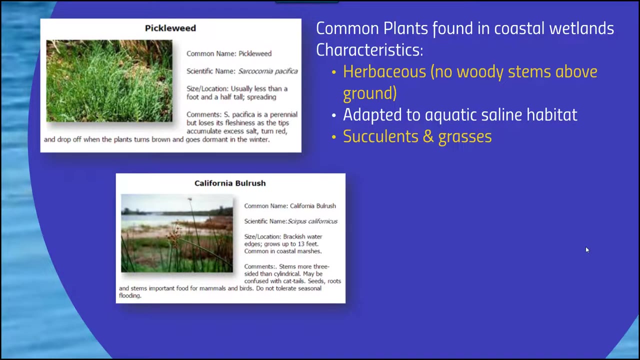 side. pickleweed is a great example you find quite commonly in San Diego. By not having that woody stem they're able to deal a lot better with these muddy or less solid soil kind of things. It's an example here of California bulrush and another one commonly found plant is salt grass. 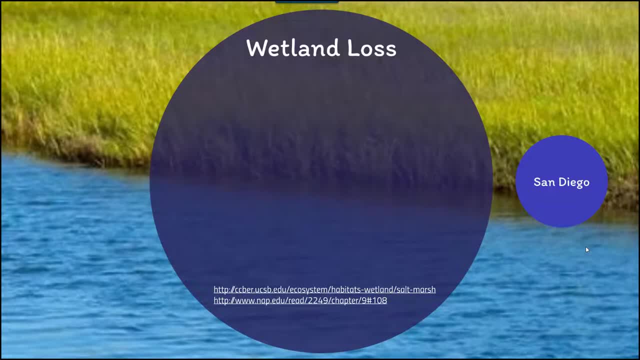 Loss of wetlands is a huge issue that we've faced within our within our coastal environments, within our coastal communities and, as I mentioned, there's a. these estuaries act as nurseries for a wide diversity of species. They also act as a filter and a buffer for flooding, as well as nutrient overloading and 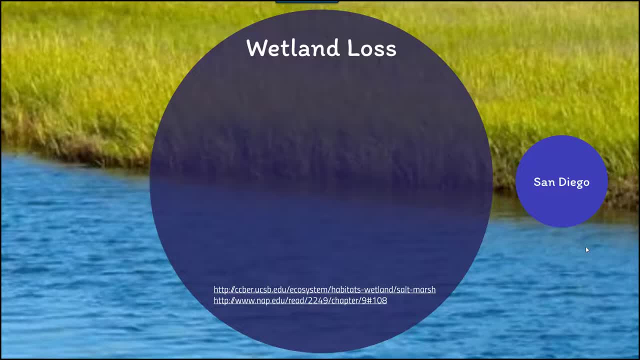 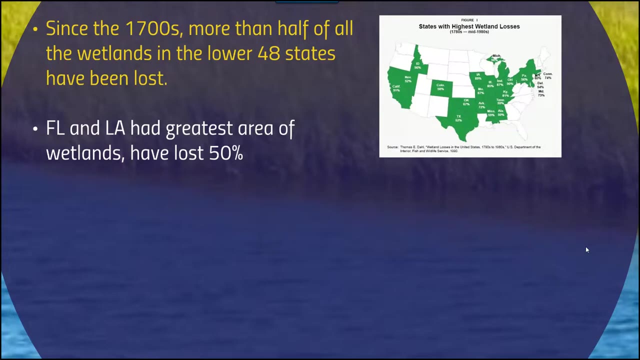 things along those lines. So the destruction of these wetlands and the loss of these habitats can be quite critical and bad for the associated and adjacent marine ecosystems. So since the 1700s there's been more than half of all wetlands in the lower 48 states lost. Florida and Louisiana had the 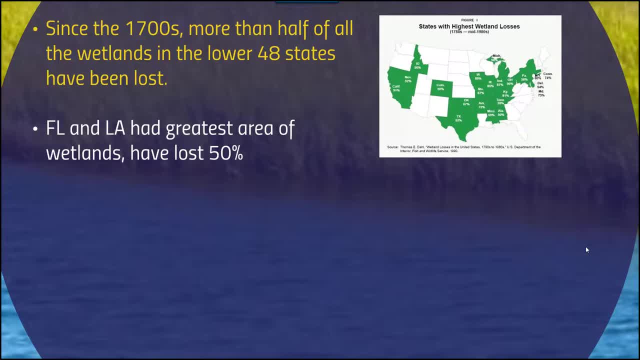 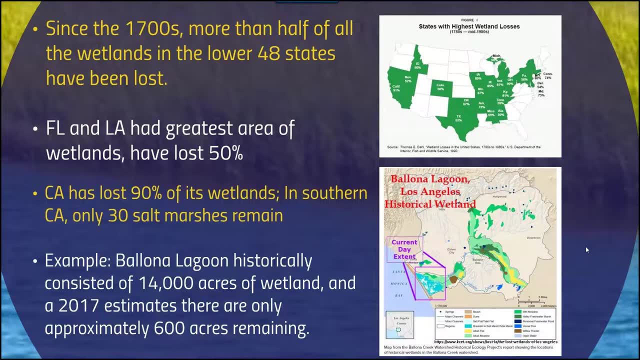 greatest area of wetlands and have lost about 50% of those, and this map over on the right-hand side indicates states with the highest wetland lost and their percentages. California has lost a little over 90% of its wetlands and in Southern California we only have 30 salt marshes remaining. 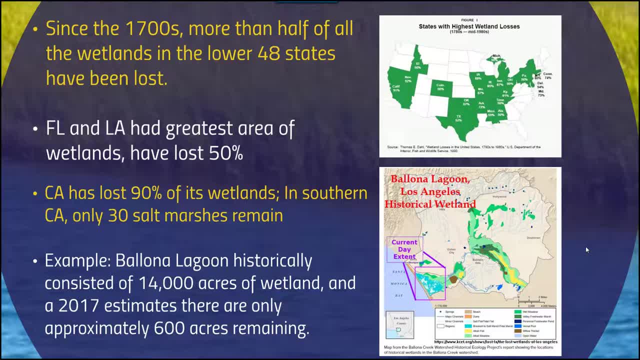 A good example of kind of the historical extent change in these wetlands is the San Diego Lagoon in Los Angeles. Historically, this wetland occurred within the entirety of this region, so this entire space was included in that wetland. Currently, though, our current day extent. 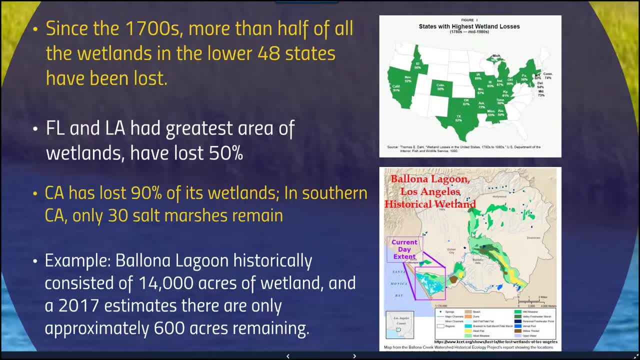 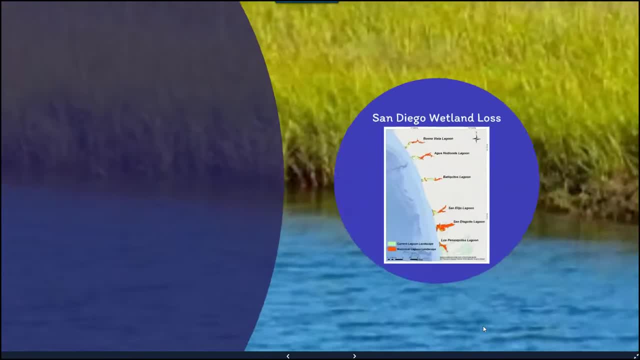 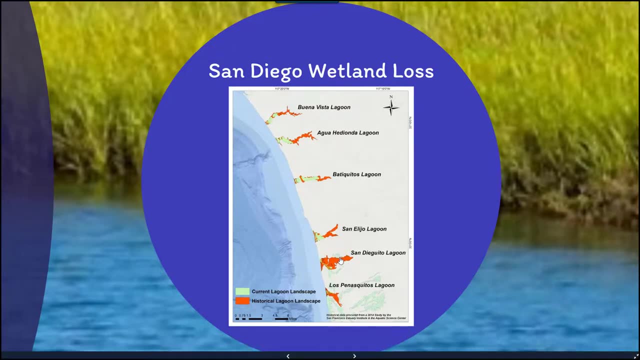 has dropped that 14,000 acres of wetland down to about 600 acres of wetland, and that was in 2017, so we've probably had a reduction since then. San Diego wetland lost is also a- you know, significant- imagine so part of the California wetland loss. If you take a look at this map, we see that the